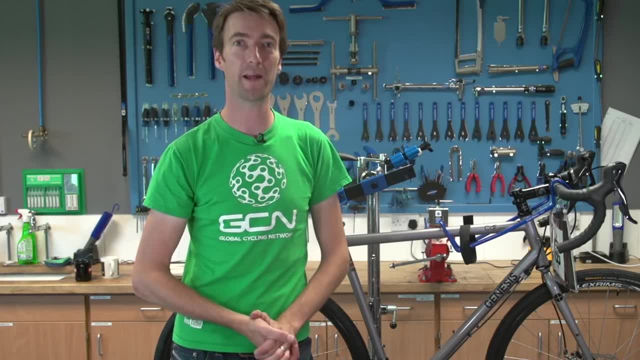 But what can you expect to get from a basic service? Well, that very much depends on how much you're willing to pay, what type of bike you've got and what type of riding you do. Now, we're assuming that, having watched our channel, 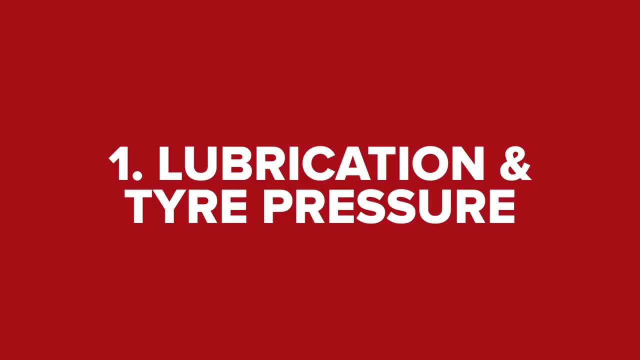 you know how to lubricate your chain and pump your tires up to the correct pressure, But if you don't- and you're a complete novice to the sport- that should be one of the first things that the bike shop checks. One thing that every bike service should include is a general safety check. 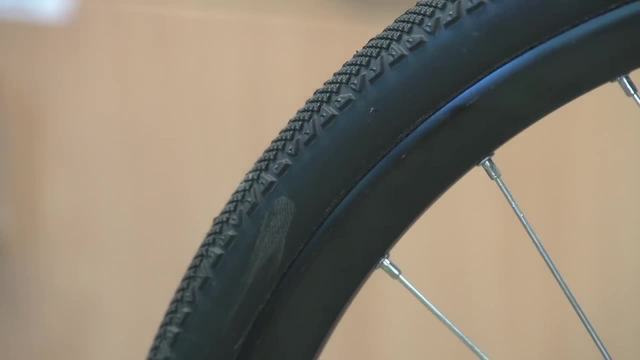 That means going over the tires, making sure the sidewalls aren't perished. there's enough grip and tread that it's not going to cause you a hazard when you're out riding. They should also go over the frame forks and the rest of the components. 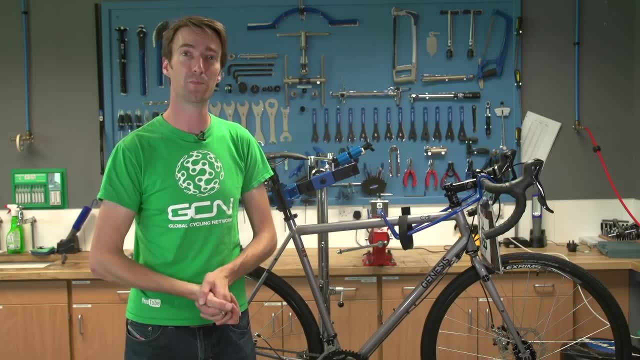 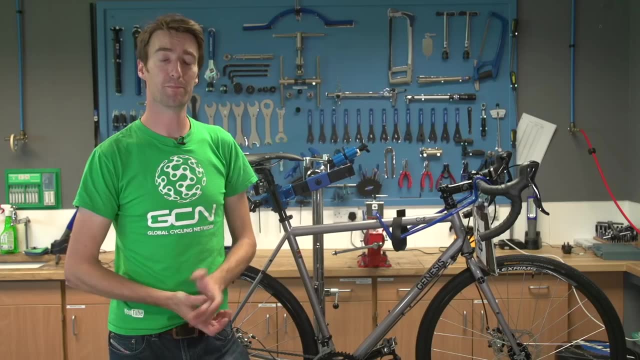 making sure there's no excessive rust or even cracks which might cause a component to fail on you whilst you're out riding. And also they'll just go over each of the bolts and make sure they're correctly tightened up. Beyond the general safety, 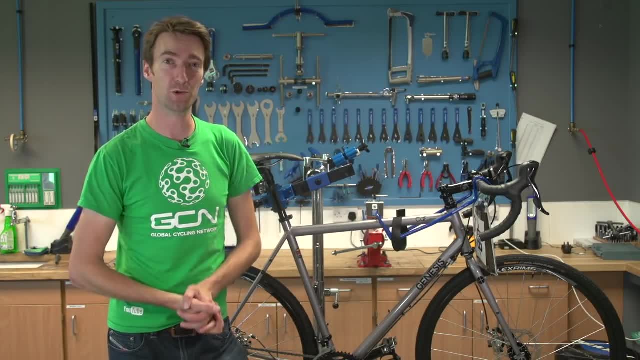 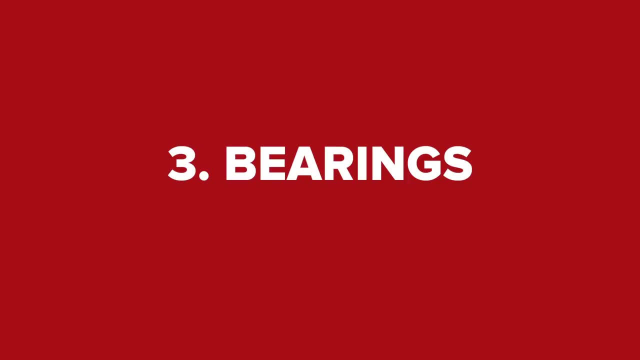 check. it's quite hard to place the next part of a bike service in order of importance, But there are a few key points that we at GCN like to make sure are regularly checked on all of our bikes. We'll start off with anything with a bearing, That means the hubs, the bottom. 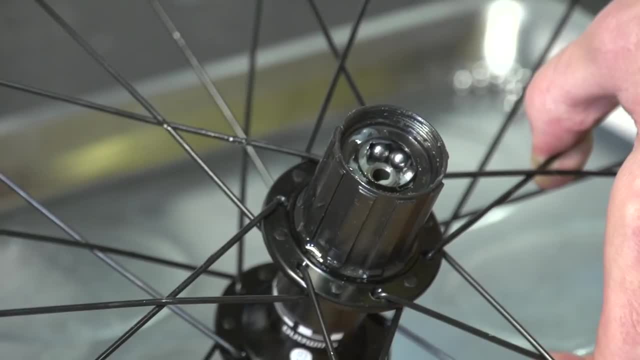 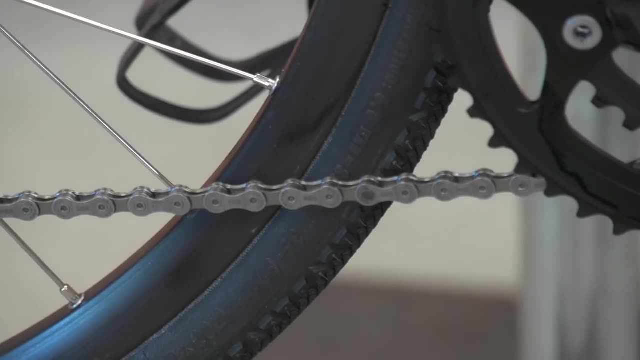 bracket and the headset. Keep them clean and well greased, and your components will be running smoothly and lasting for longer. Same goes for the chain. That wears very quickly on any bike if you use it regularly. Replace that often and in the long run you'll save money because a stretch chain will wear both. 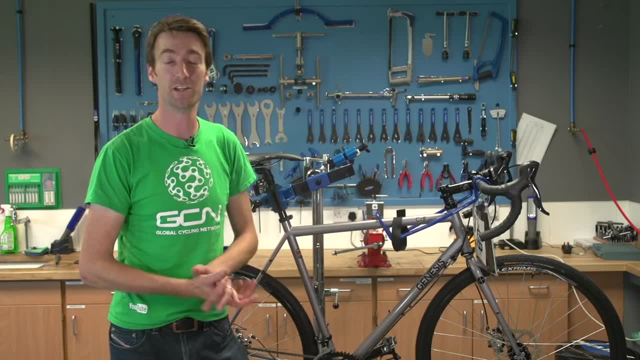 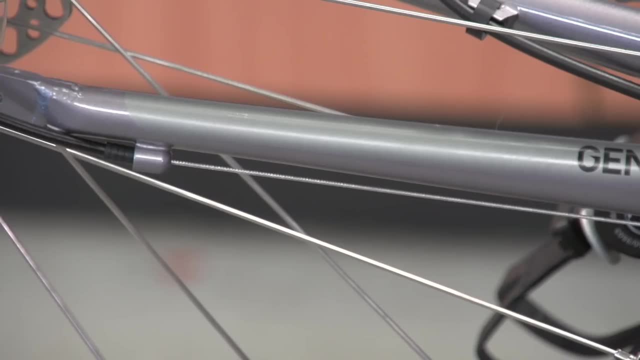 the chains at the front and the cassette at the rear, and that means that you could end up having to replace the whole lot. On to cables now, and it's amazing how quickly you get used to riding with old, mucky or even frayed. 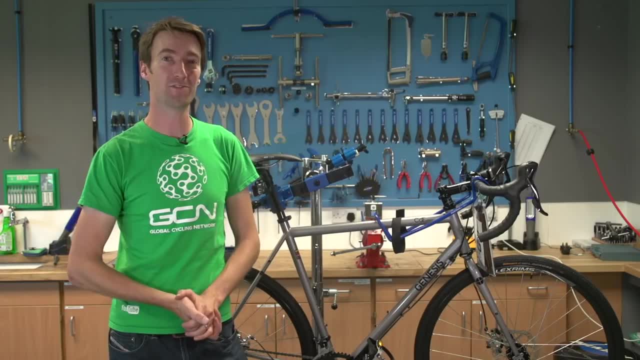 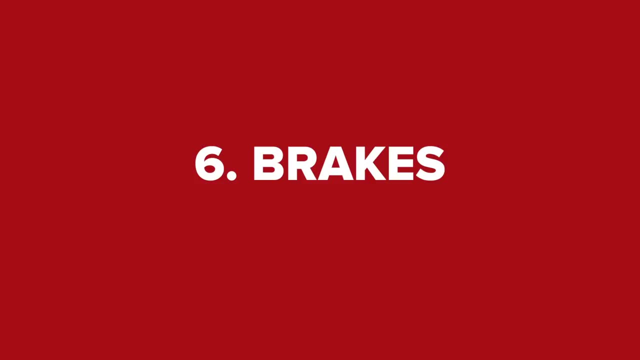 cables, which of course don't work very efficiently, And you'd be surprised at how different your bike feels if you replace both the inners and outers of the gears and brakes. And talking of brakes, the bike shop should also check the brake pad wear. It doesn't matter if you're using disc brakes or rim brakes. 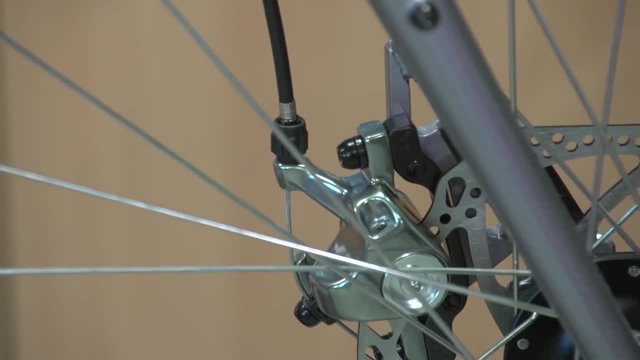 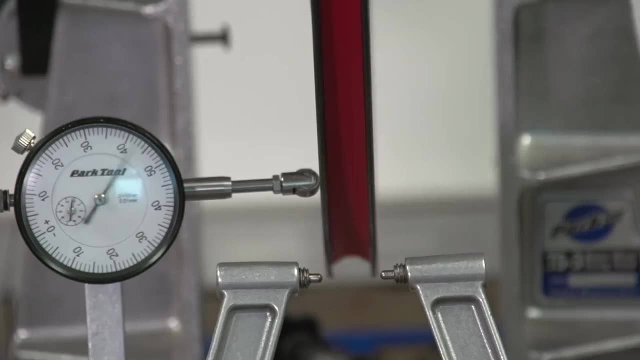 the pads get down too low, you risk going down to metal on metal, which of course doesn't offer a great deal of stopping power. On to the wheels now, and if you've got a slight buckle in one or both of them, it shouldn't take a good bike shop.